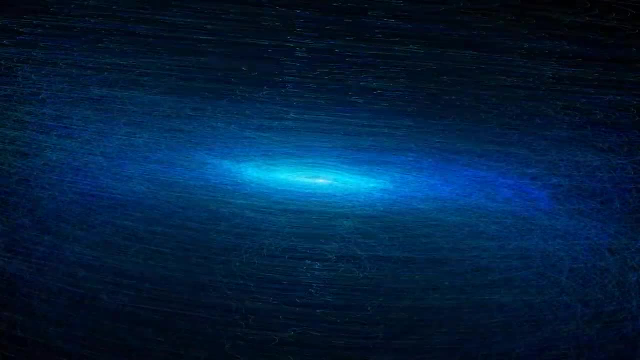 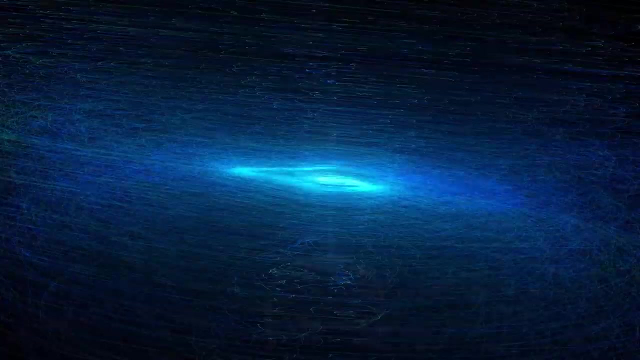 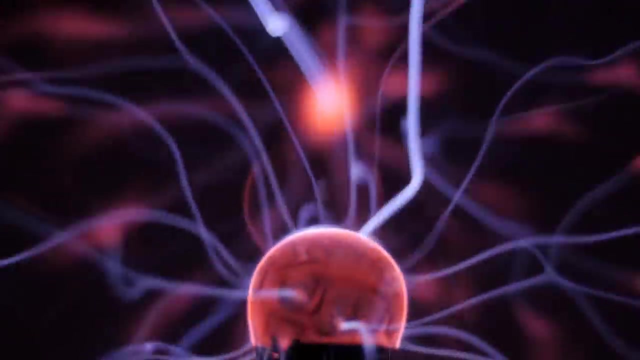 Hi, let's play a game and see what's your electromagnetic knowledge. I will ask you some questions. After that you should pause the video and think about the answers, Then go on and see the real answer Ready. First one: Do you know what electromagnetism is? Electromagnetism- 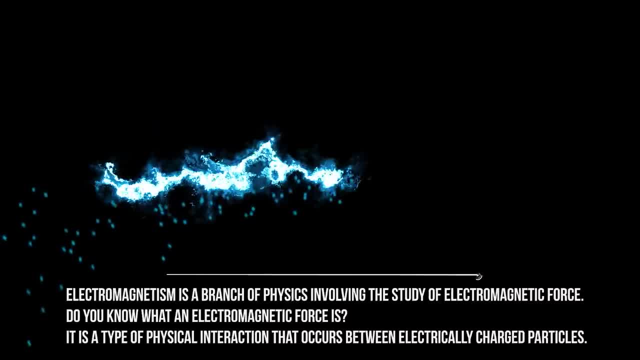 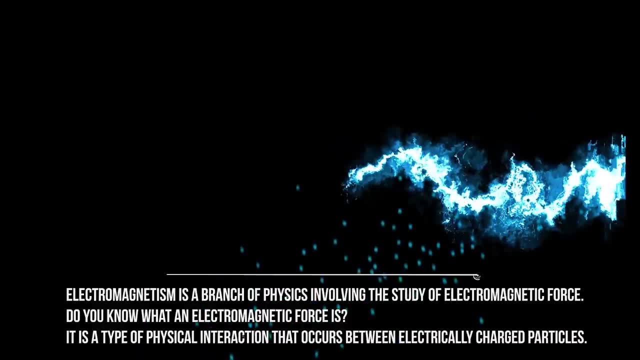 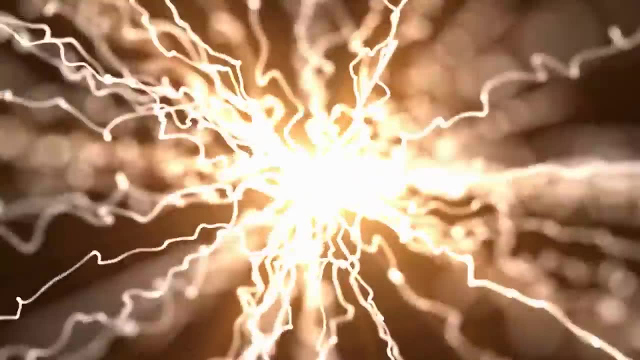 is a branch of physics involving the study of electromagnetic force. Do you know what an electromagnetic force is? It's a type of physical interaction that occurs between electrically charged particles. Well, do you know what electrically charged particles are? I bet you. 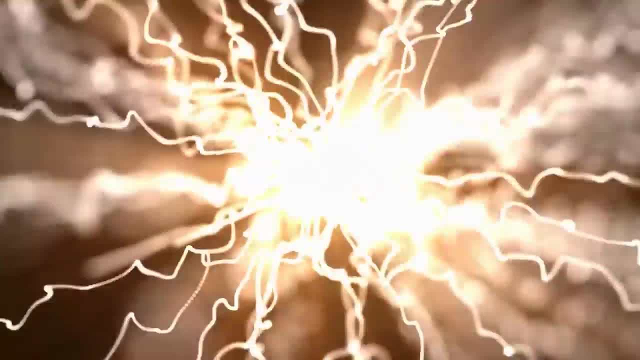 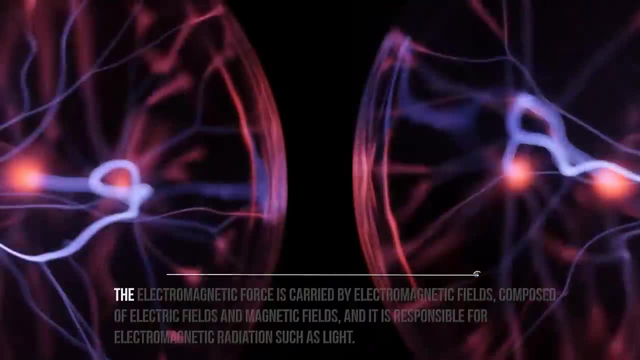 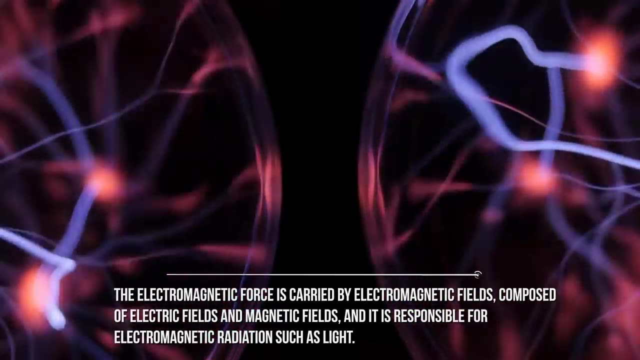 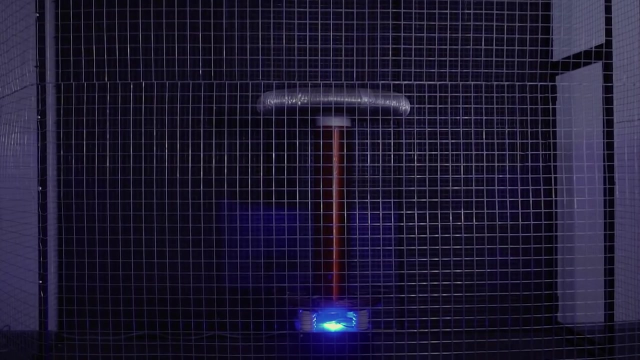 know some of them, such as protons and electrons. The next question could be: what carries the electromagnetic force? The electromagnetic force is carried by electromagnetic fields composed of electromagnetic forces. The electromagnetic force is carried by electromagnetic forces. It is responsible for electromagnetic radiation such as light. Wait, what Is light? a type of 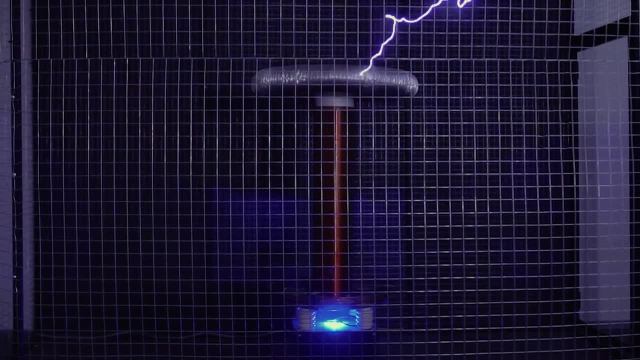 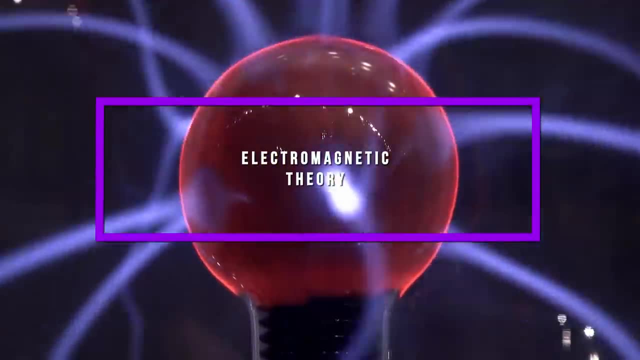 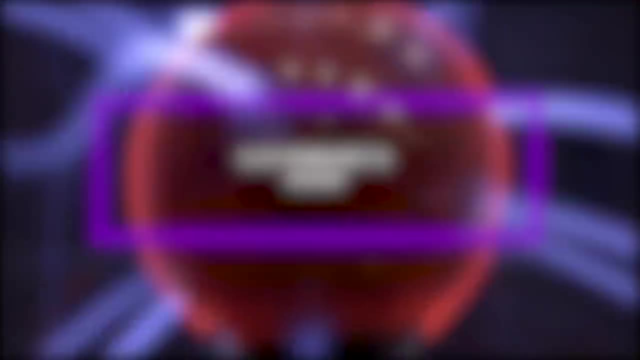 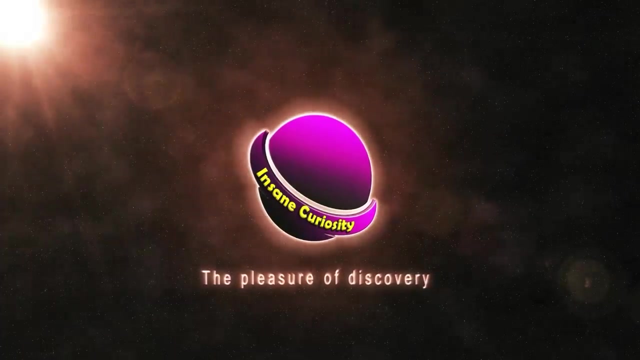 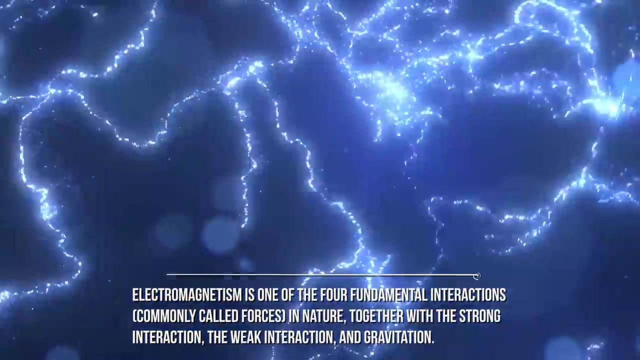 electromagnetic radiation. We will get back to it later in this video. I'm glad you decided to play with us Now. if you want to take things more seriously and interesting, we suggest you keep watching this video about electric and magnetic theory. Electromagnetism is one of the four fundamental interactions commonly called forces in nature. 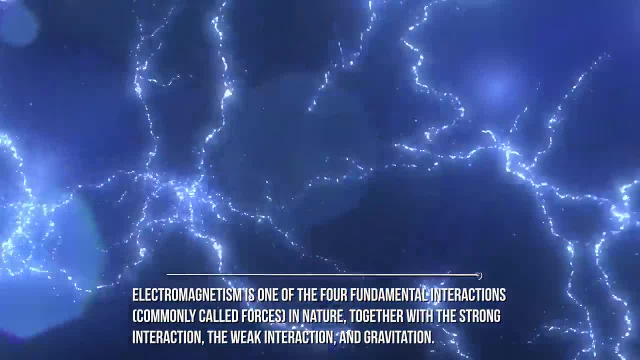 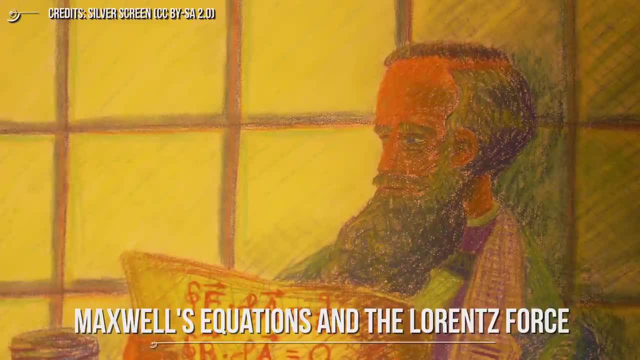 together with the strong interaction, the weak interaction and gravitation. The laws that lie behind electromagnetic phenomena are elegant. They are the so-called Maxwell's equations and the Lorentz force. Actually, the Lorentz force is the law of the universe, It is the law of the 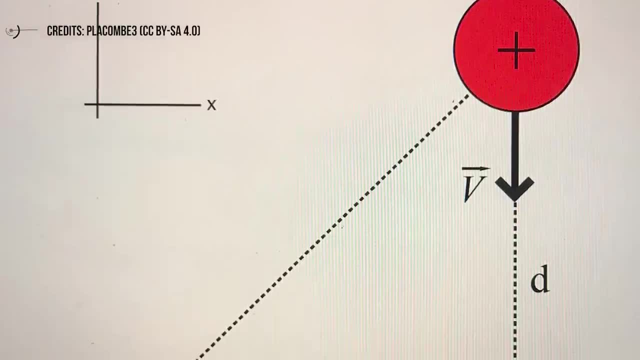 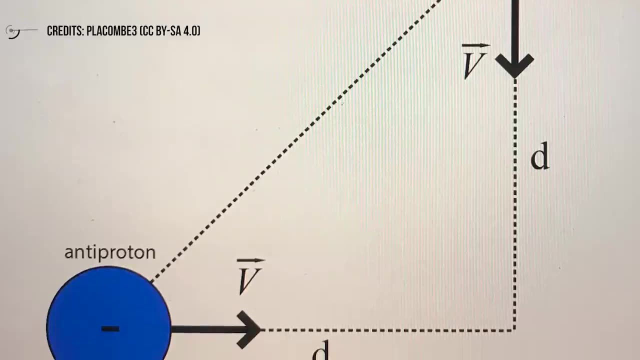 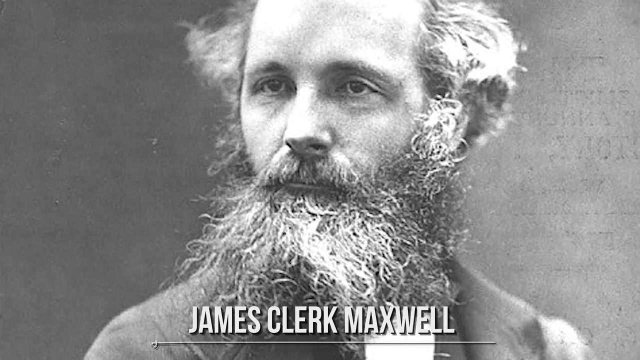 universe. In fact, there are numerous mathematical descriptions of the electromagnetic field, and Maxwell's equations describe how electric and magnetic fields are generated and altered by each other and by charges and currents. Maxwell was an insane thinker and scientist. His theoretical and observational work led 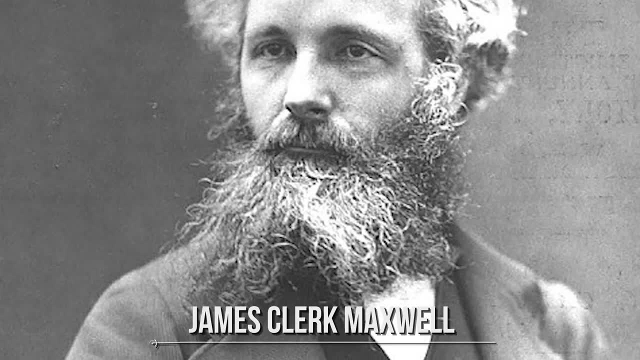 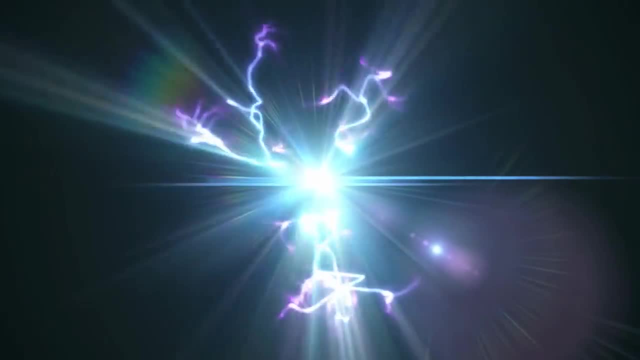 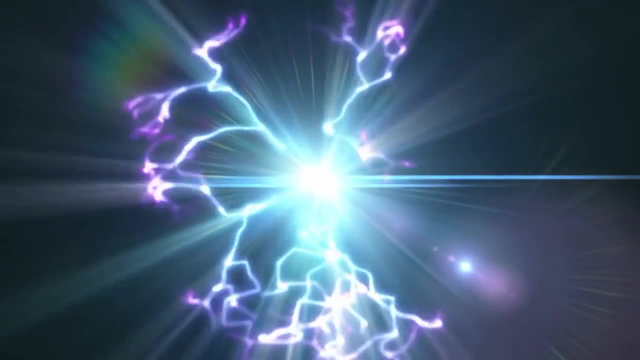 to the development of special relativity by Albert Einstein in 1905.. In fact, Maxwell saw that electromagnetic waves go through space at the speed of light. This was a crucial result that entered, amazingly, in the special relativity theory. But let's go back in time and see how we got there. 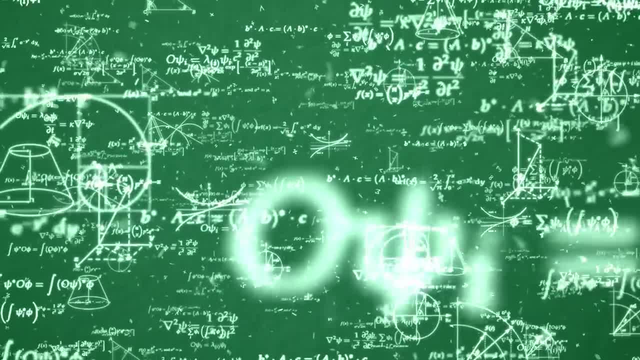 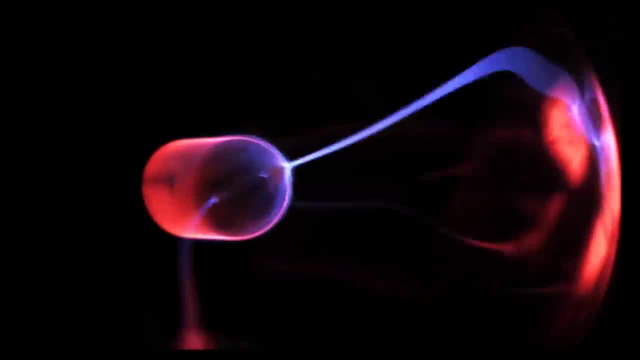 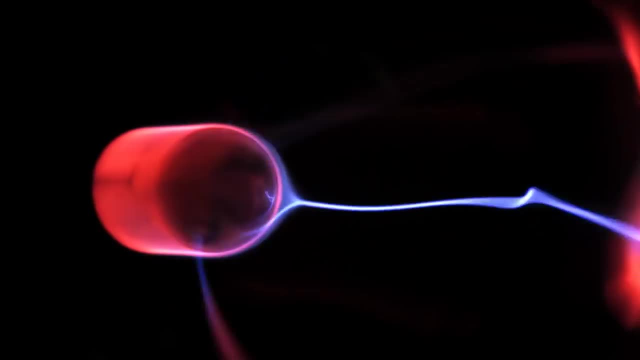 What did the world know about electromagnetic theory before Maxwell? What were the first electromagnetic phenomena ever observed and studied? Long before any knowledge of electromagnetism existed as a concept, people were aware of the effects of electromagnetic' of electricity. Now we know that we can think of electromagnetism as a combination of electricity. 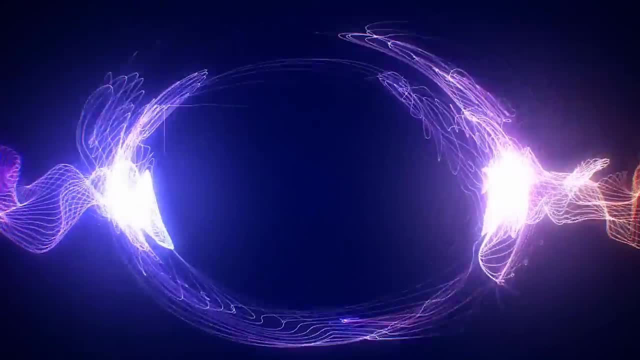 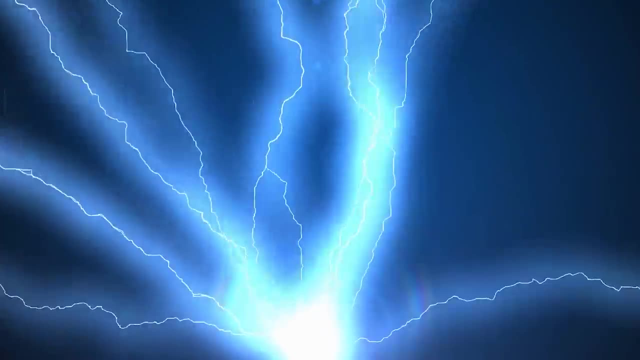 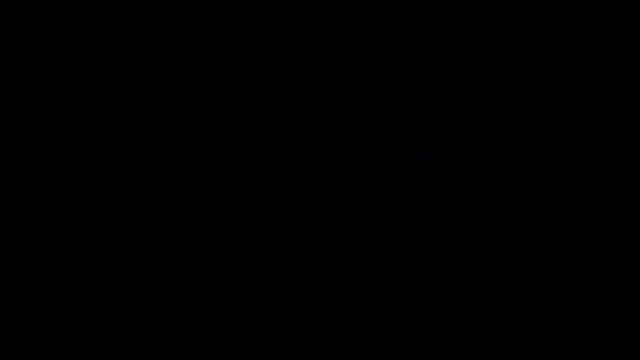 and magnetism, but people at the time thought they were two distinct things that had nothing to do with each other. Lightning and other manifestations of electricity were known in ancient times, but it was not understood that these phenomena had a common origin. One possible approach to the discovery of the identity of lightning and electricity: 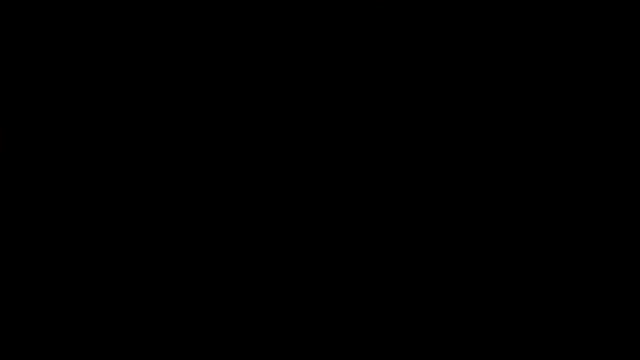 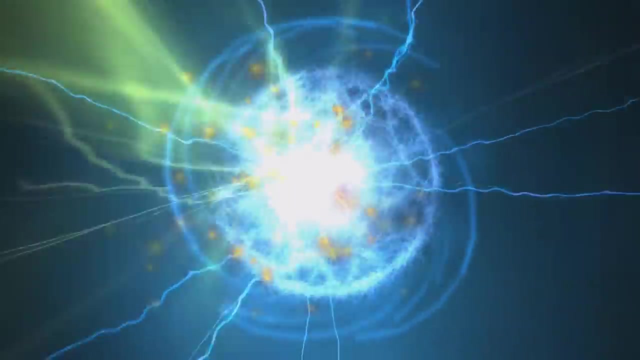 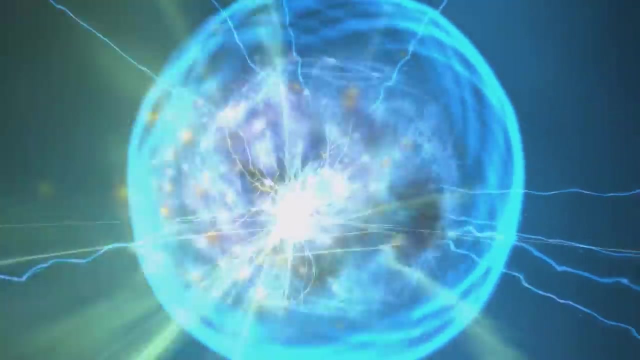 is to be attributed to the Arabs who, before the 15th century, used the same Arabic word for lightning and the electric ray. Thales of Miletus noted that rubbing fur on various substances such as amber would cause them to attract specks of dust and other light objects. 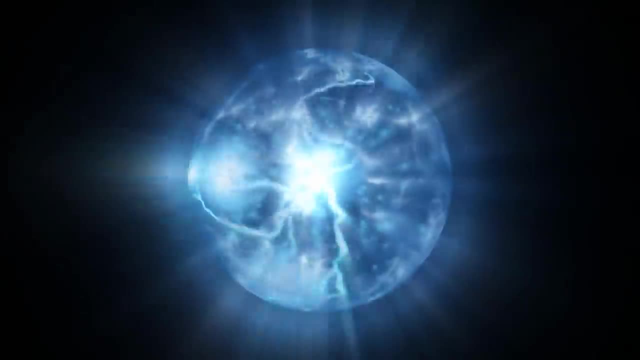 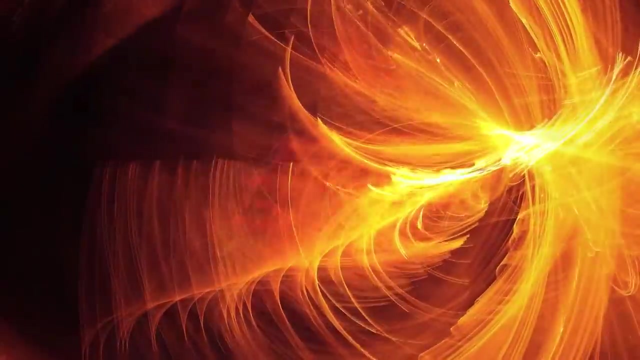 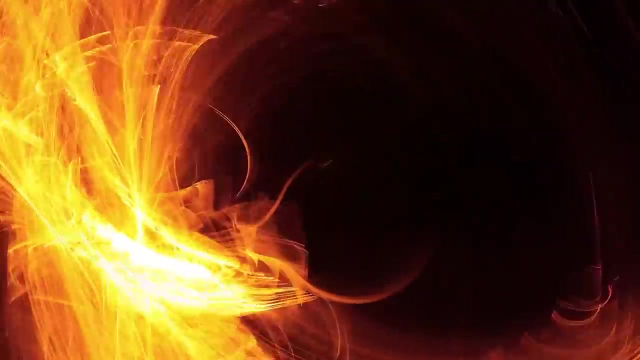 Thales wrote on the effect now known as static electricity. The Greeks noted that if they rubbed the amber for long enough, they could even get an electric spark to jump. Electrostatic phenomena were also reported millennia later by Roman and Arabic naturalists and physicians. It was no magical trick. it was a new phenomenon that begged to be studied. 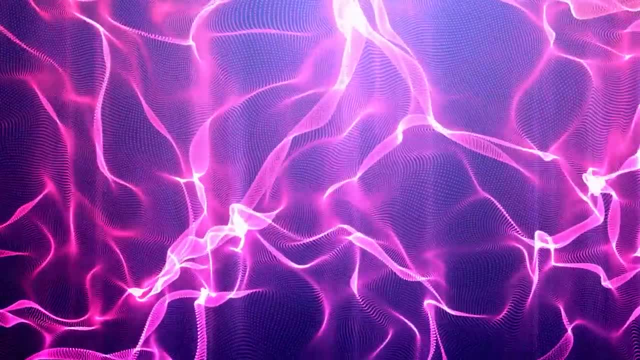 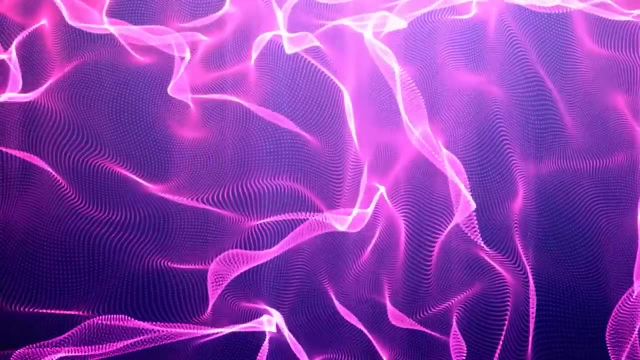 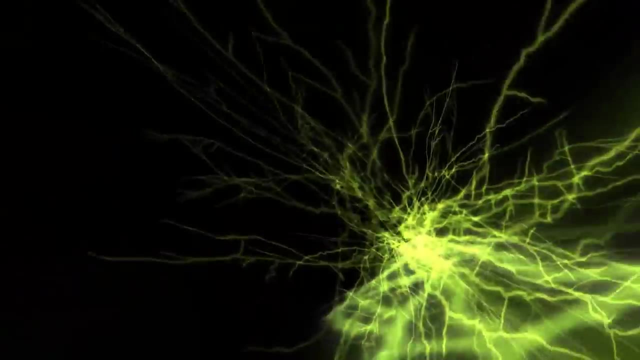 Just to understand the importance of electromagnetic theory, that the electromagnetic force is responsible for practically all phenomena one encounters in daily life above the nuclear scale, with the exception of gravity. Roughly speaking, All the forces involved in interactions between atoms can be explained by the electromagnetic 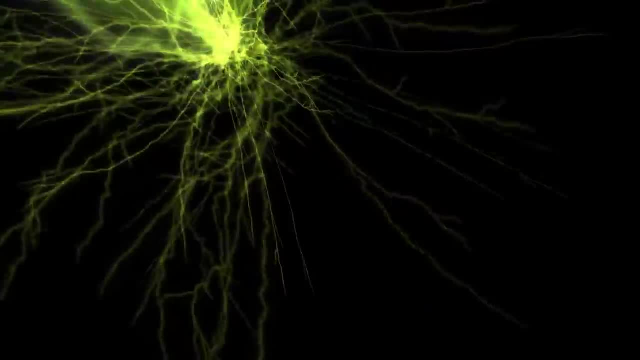 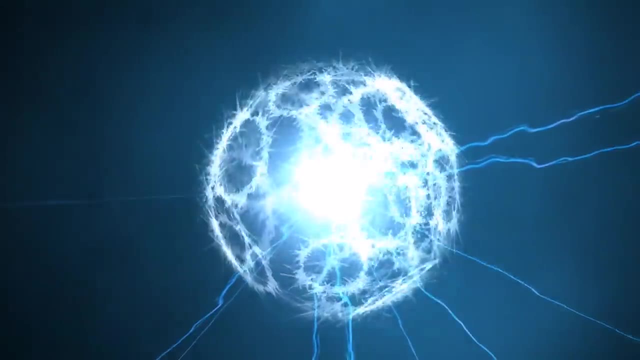 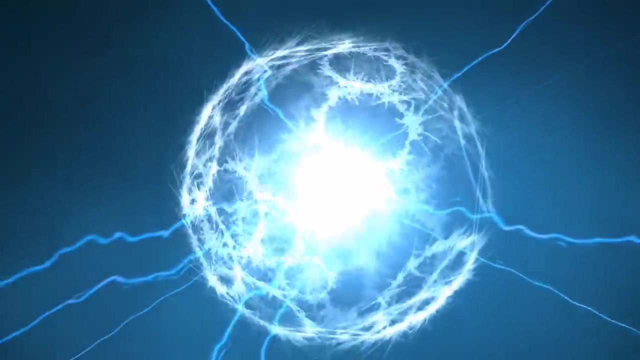 force acting between the electrically charged atomic nuclei and electrons of the atoms. Electromagnetic forces also explain how these particles carry momentum by their movement. This includes the forces we experience in pushing or pulling ordinary material objects, which result from the intermolecular forces that act between the individual molecules. 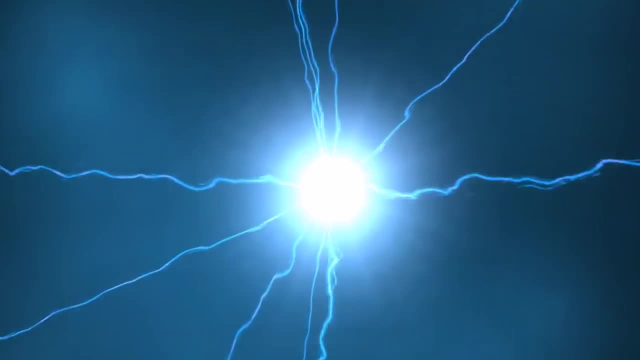 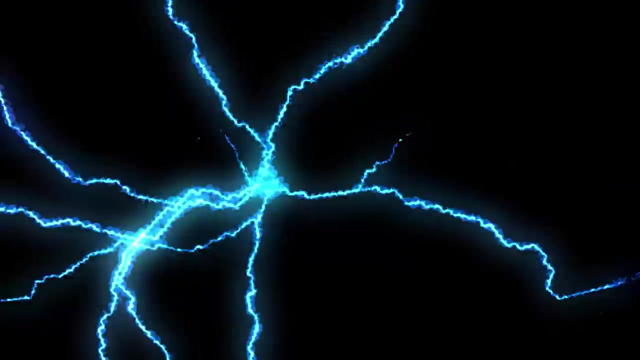 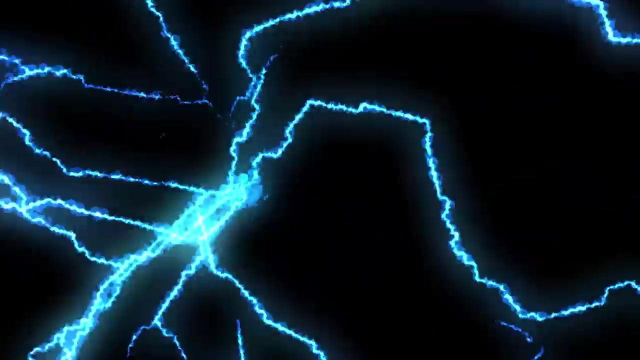 in our bodies and those in the objects. The electromagnetic force is also involved in all forms of chemical phenomena. People didn't know any of that, but with time someone started to feel that there was much at stake. The first remarkable in-depth study of electric and magnetic phenomena as a whole started. 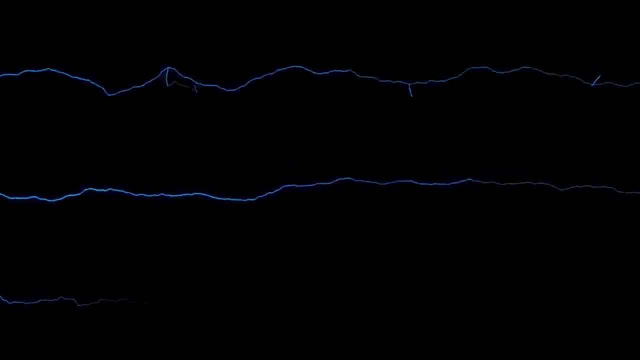 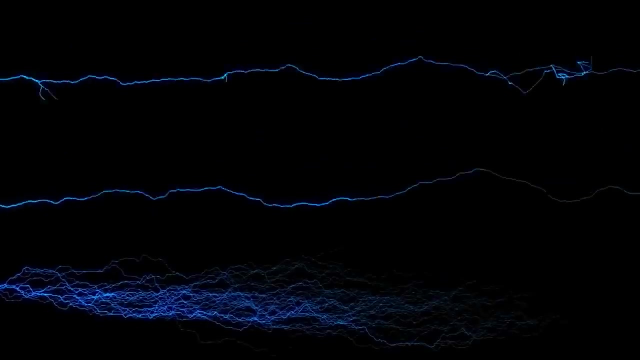 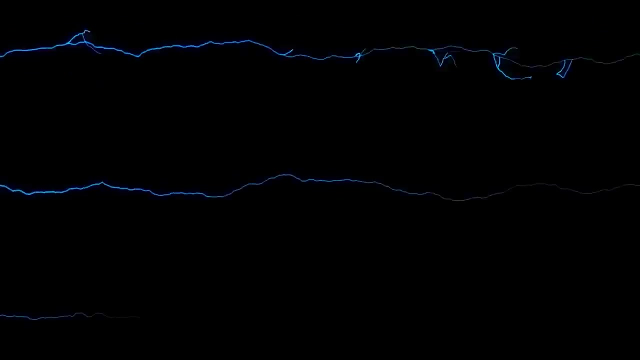 around 1800.. In April 1820, scientist Hans Christian Ørsted observed that an electrical current would move in the direction of an electron. The current in a wire caused something strange: A nearby compass needle was moving Again, it was no magical trick, it was justscience. 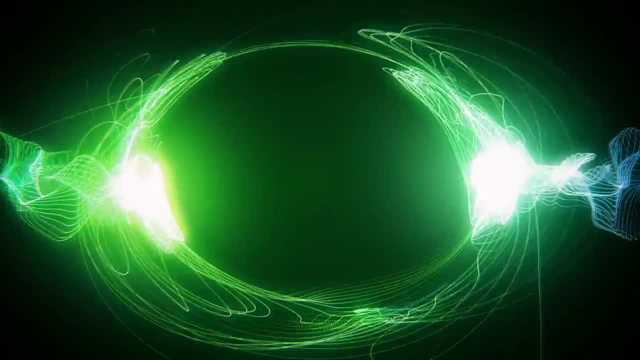 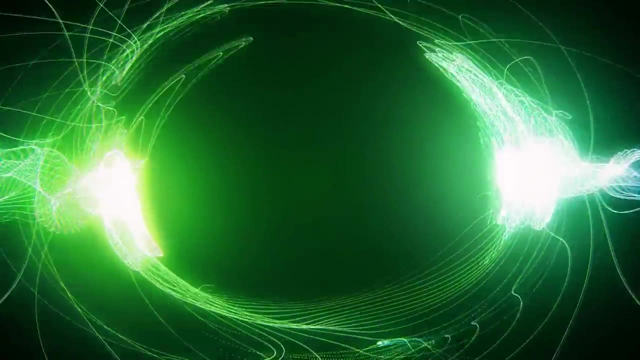 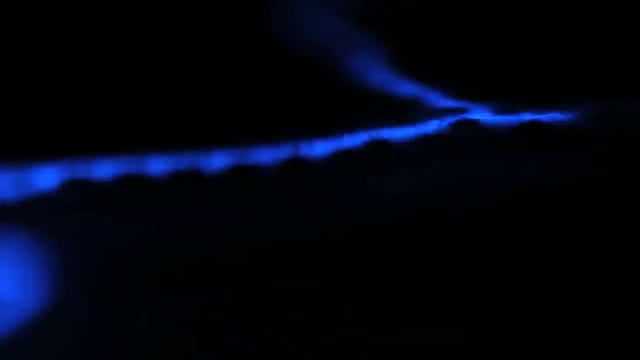 Did he know that? Yes, and at first he struggled in order to find a satisfactory explanation of the phenomenon, but he could not find it. Also, he didn't try to represent the phenomenon in a mathematical framework. however, three months later, he began more intensive investigations. 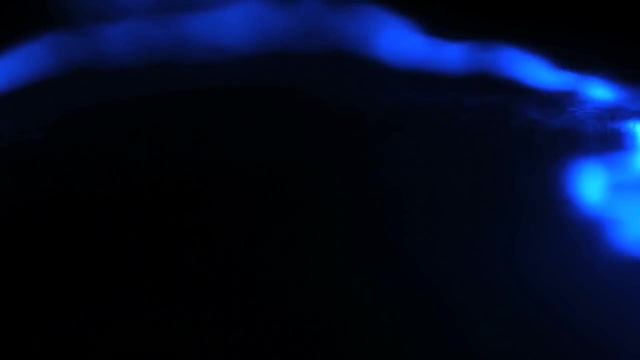 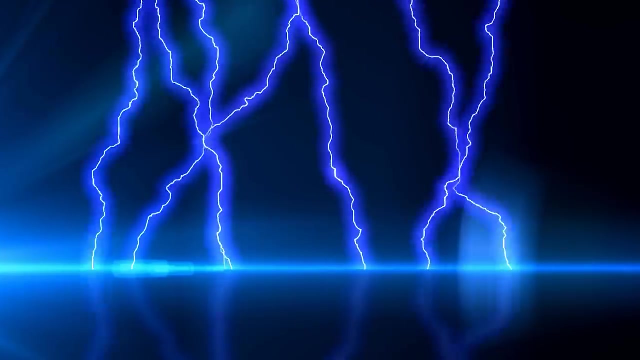 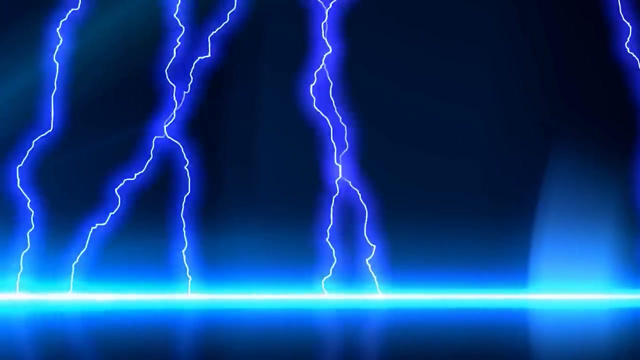 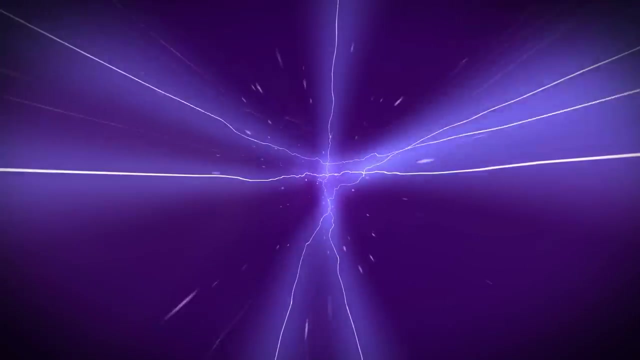 This led to the publishing of his findings proving that an electric current produces a magnetic field as it flows through a wire. That's why the CGS unit of magnetic induction is today named Ørsted. He literally got what he deserved. After that, Ørsted's findings resulted in intensive research throughout the scientific 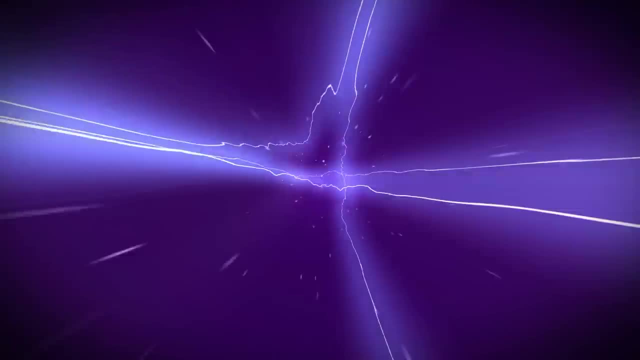 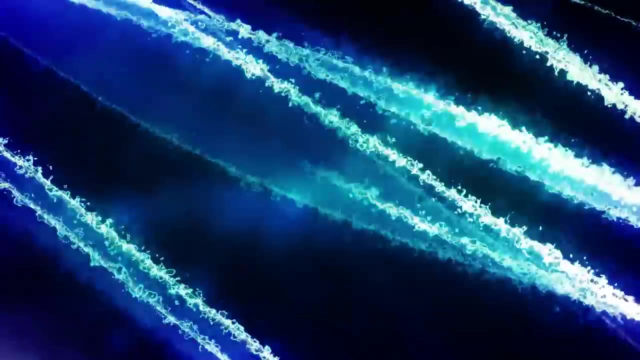 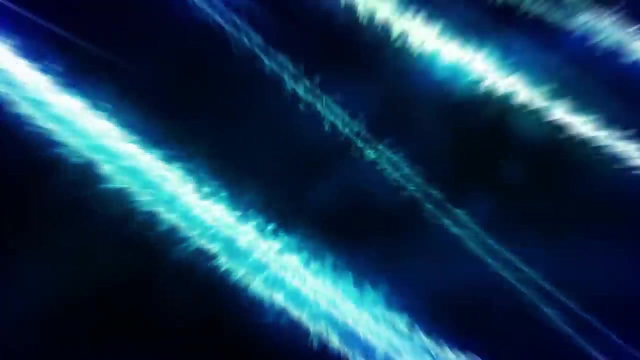 community. They influenced French physicist Ampere's developments of a mathematical theory In the early 19th century. Ørsted used a mathematical form to represent the magnetic forces between current-carrying conductors. Ørsted's discovery also represented a major step toward a unified concept of energy. 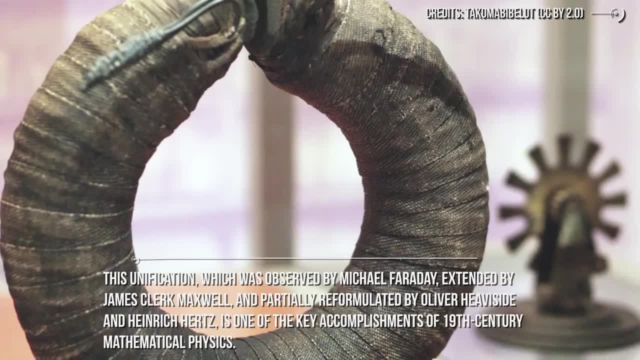 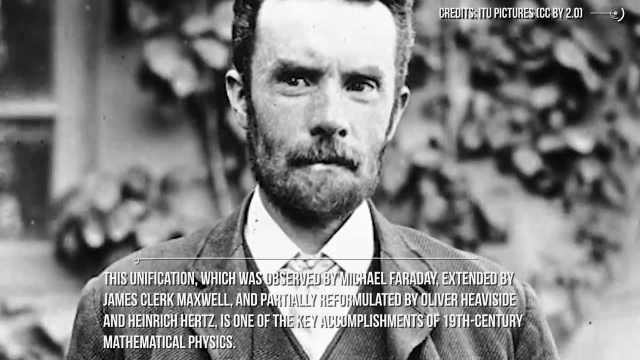 This unification, which was observed by Michael Faraday, extended by James Clerk Maxwell and partially reformulated by Oliver Heaviside and Heinrich Hertz, is one of the key accomplishments of 19th century mathematical physics In particular. things really changed. 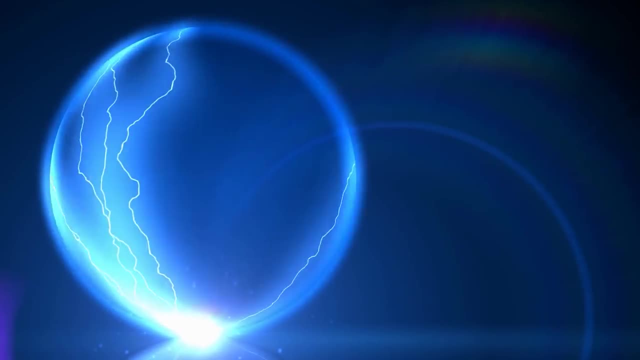 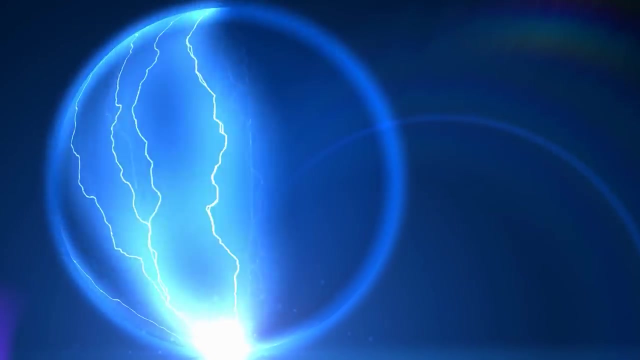 The first thing that happened in 19th century was that the magnetic force of the current current-carrying conductors changed. This changed with the publication of James Clerk Maxwell's 1873 A Treatise on Electricity and Magnetism, in which the interactions of positive and negative charges were shown. 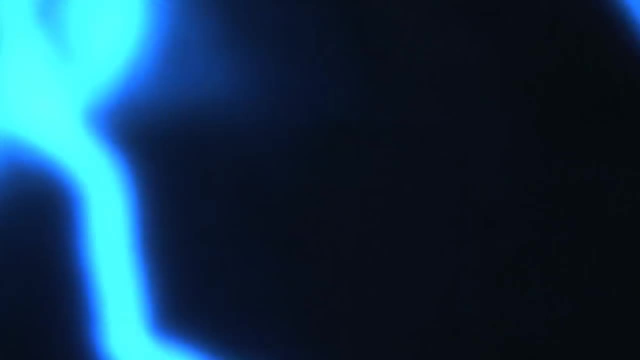 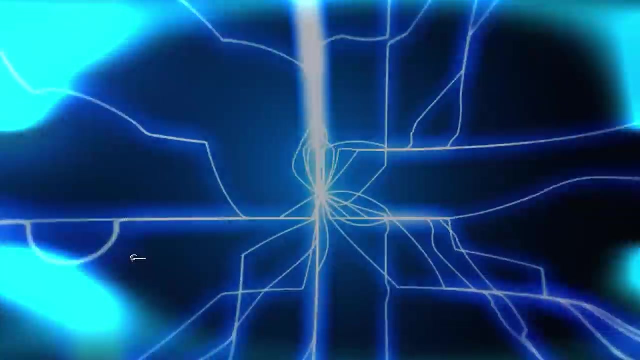 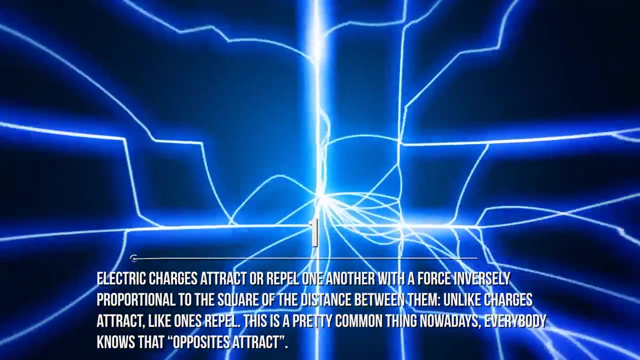 to be mediated by one force. There are four main effects resulting from these interactions, all of which have been clearly demonstrated by experiments. 1. Electric charges attract or repel one another with a force inversely proportional to the square of the current current. 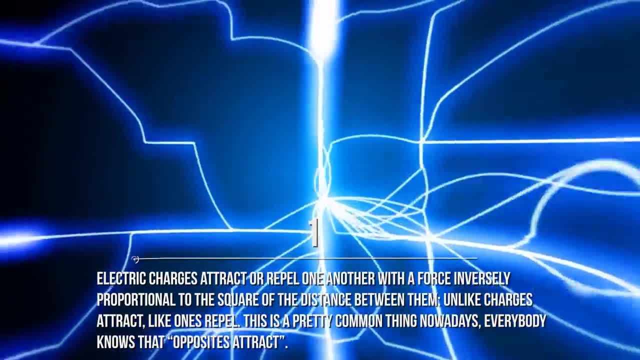 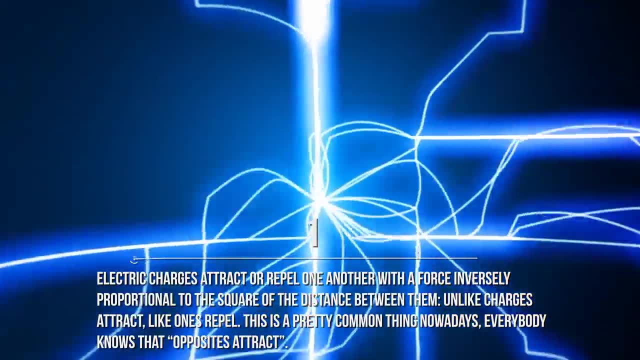 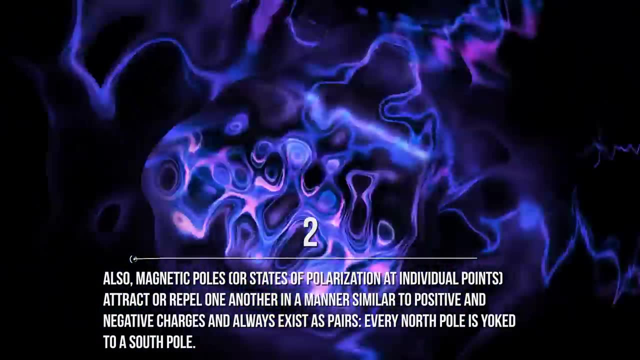 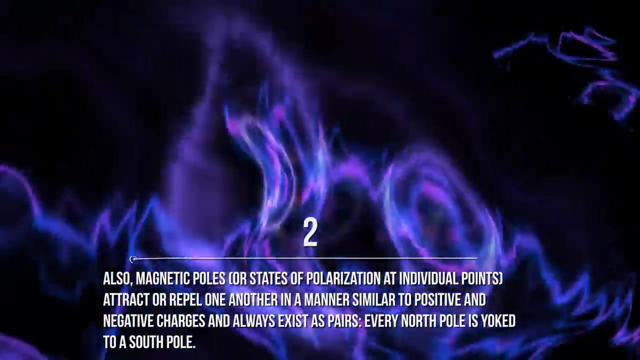 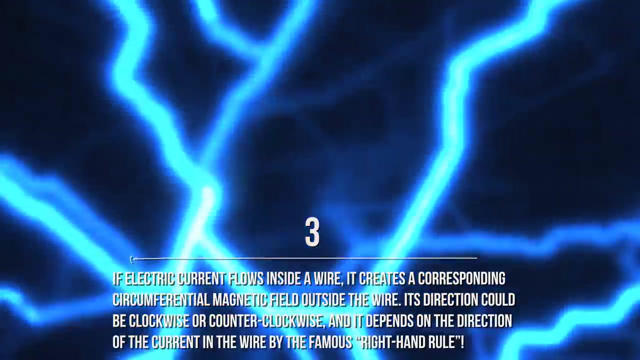 2. Magnetic poles or states of polarization at individual points attract or repel one another in a manner similar to positive and negative charges and always exist as pairs. Every north pole is yoked to a south pole. 3. If electric current flows inside a wire, it creates a corresponding circumferential magnetic 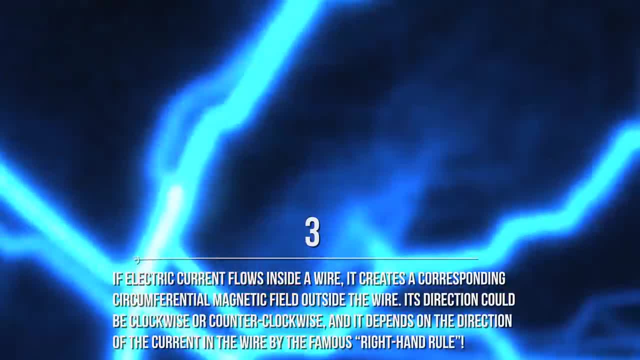 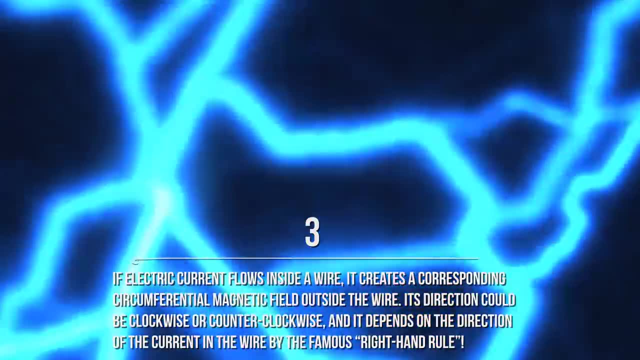 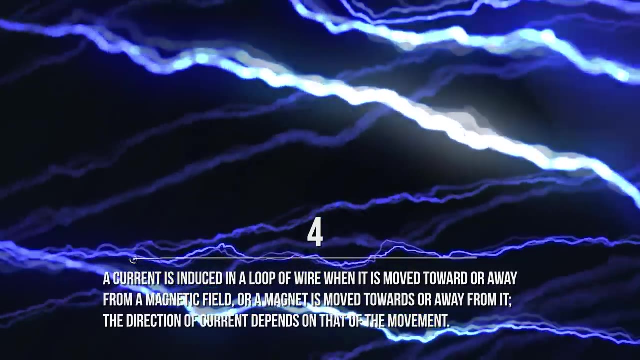 field outside the wire. Its direction could be clockwise or counterclockwise and it depends on the direction of the current in the wire by the famous right-hand rule 4.. A current is induced in a loop of wire when it is moved toward or away from a magnetic. 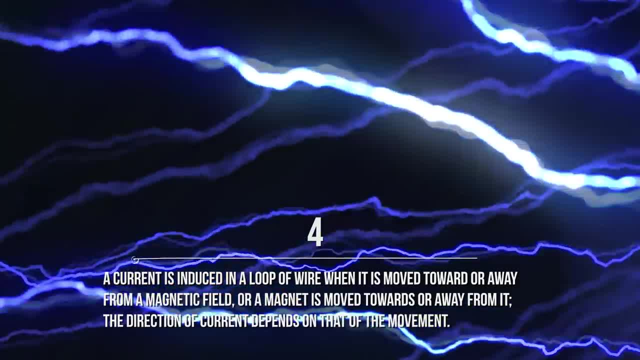 field or a magnet is moved toward or away from it. The magnetic field or a magnet is moved toward or away from it. The magnetic field or a magnet is moved toward or away from it. The direction of the current depends on that of the movement. 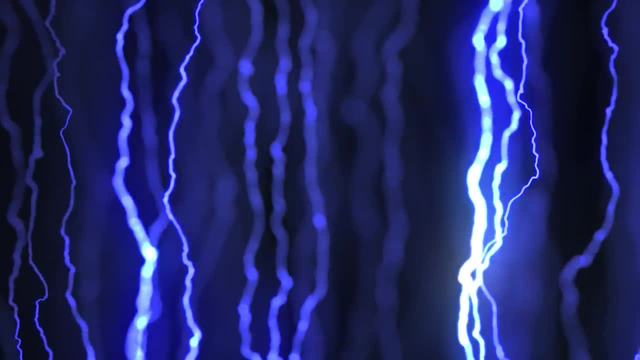 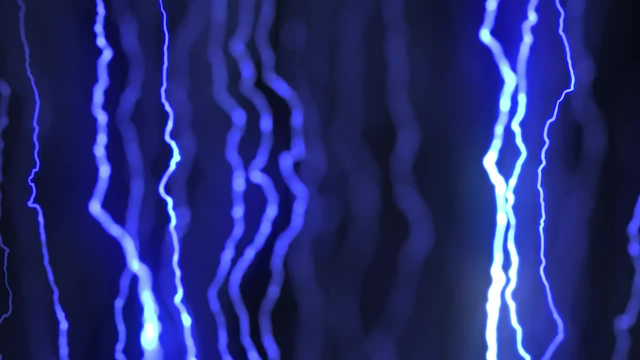 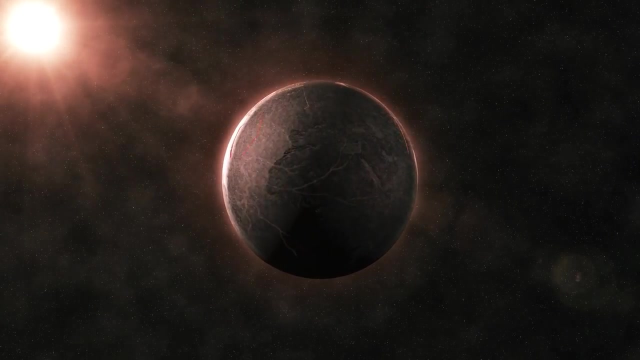 All of this has had far-reaching consequences, one of which was the understanding of the nature of light. The understanding of the nature of light is perhaps one of the most important things in all physics history. Do you want to know why? Before finding the answer to this question, be sure to like or dislike the video, so that 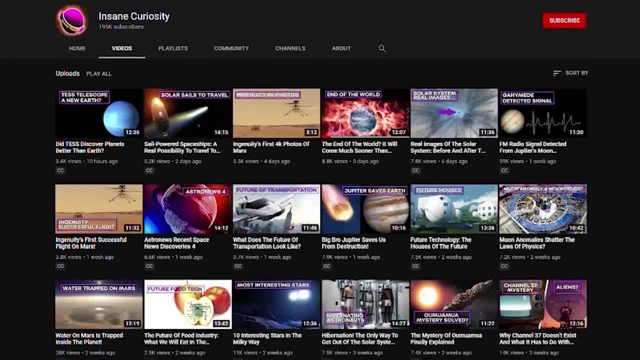 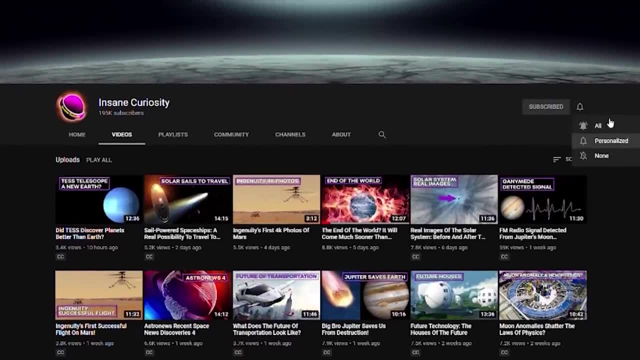 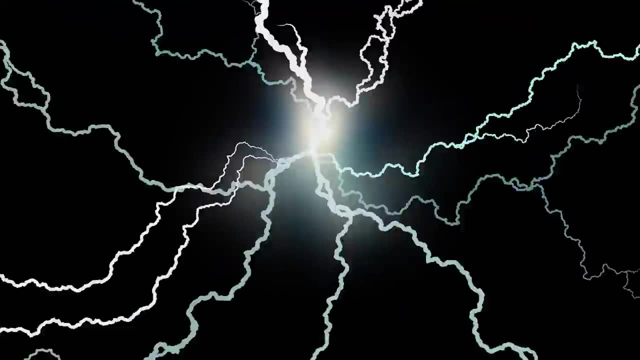 we can continue to improve and make these videos better for you and your family. Plus, be sure to subscribe to the channel by clicking the bell so that you don't miss any of our weekly videos. The answer is pretty simple but subtle. When we discovered that light was nothing but an electromagnetic wave, we had a mathematical 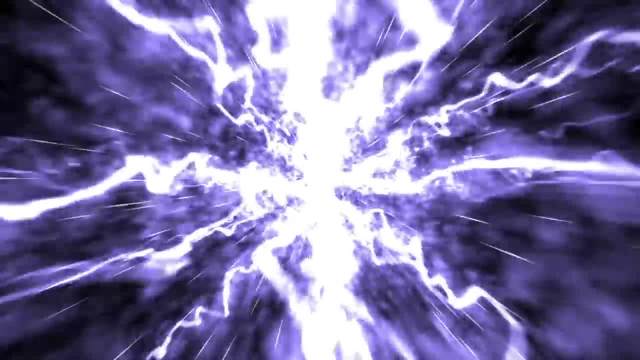 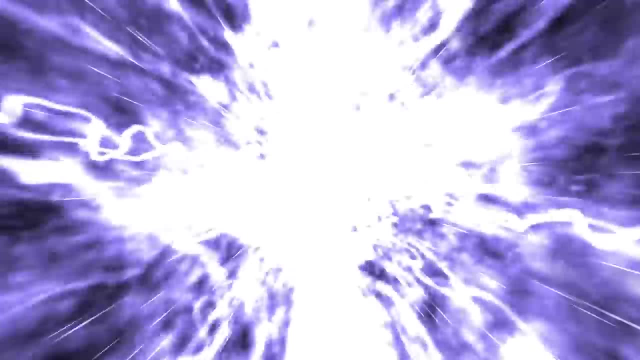 framework to treat it. For example, we know how to describe the speed of an electromagnetic wave, and Maxwell found that all of the electromagnetic waves traveled at a velocity of about 3.5 kilometers per second, That's about 300,000 kilometers per second in a vacuum. 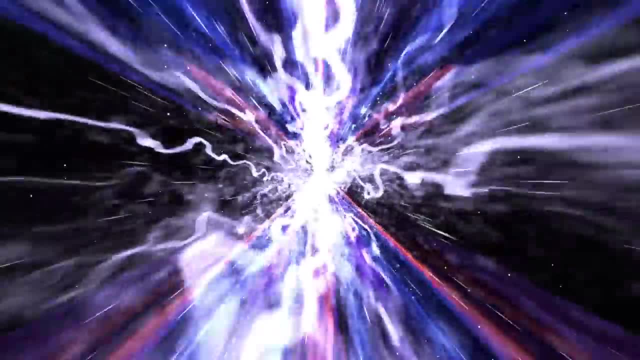 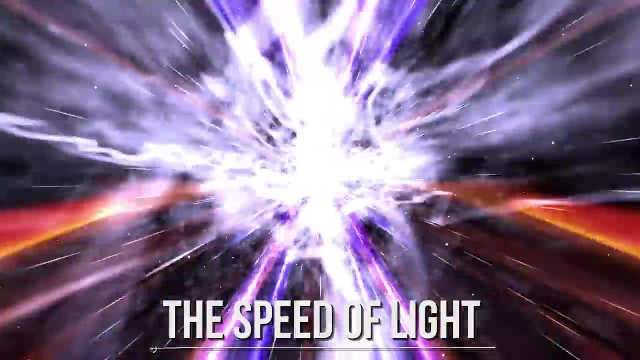 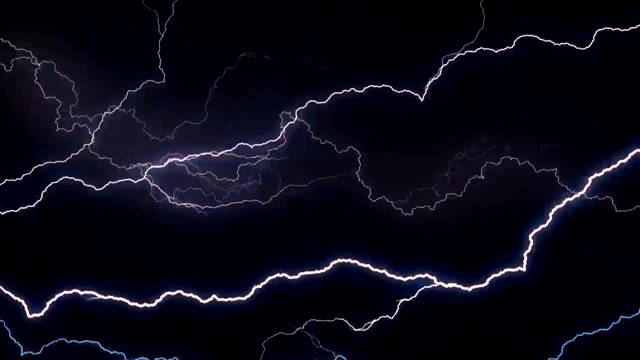 Once scientists found that light was an electromagnetic wave, the game was made. Even the light was traveling at that peculiar velocity. that's why we call it the speed of light. Also, the nature of light has always been controversial. Today we know that photons which made up the light can actually behave as waves or 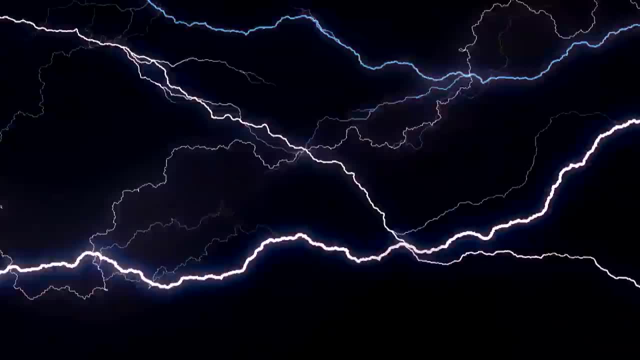 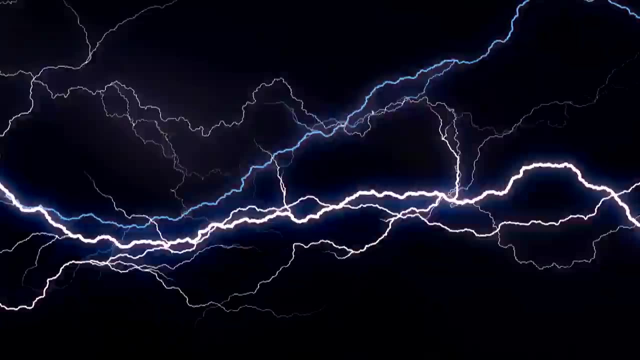 as particles. In fact, we know that photons, which made up the light, can actually behave as waves or as particles. In fact, unlike what was proposed by the electromagnetic theory of that time, light and other electromagnetic waves are at present seen as taking the form of quantized self-propagating oscillatory. 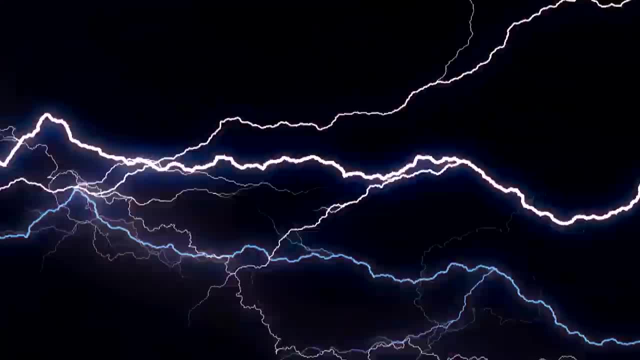 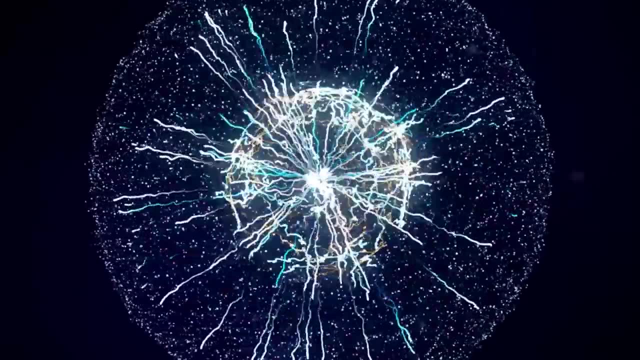 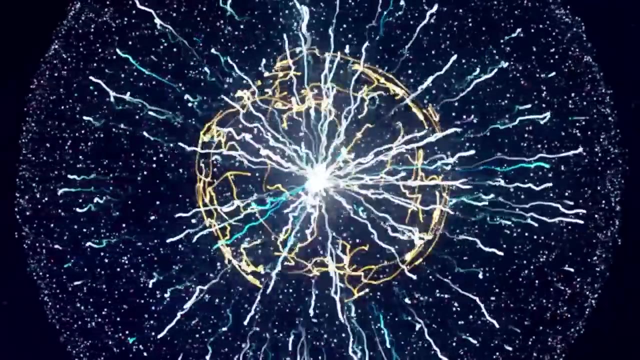 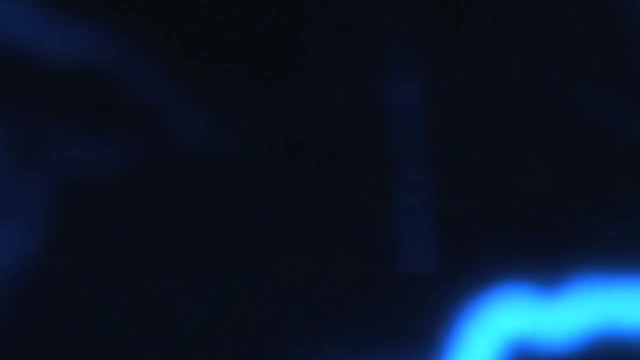 electromagnetic field disturbances called photons. Different frequencies of oscillation give rise to the different forms of electromagnetic radiation, from radio waves at the lowest frequencies to visible light at intermediate frequencies to gamma rays at the highest frequencies. Anyway, taking into account quantum behaviors would be too much for the purpose of this. 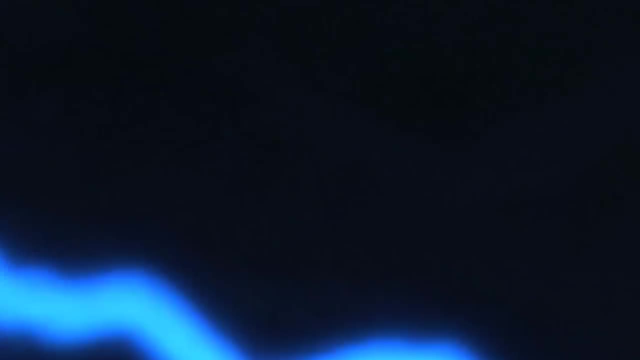 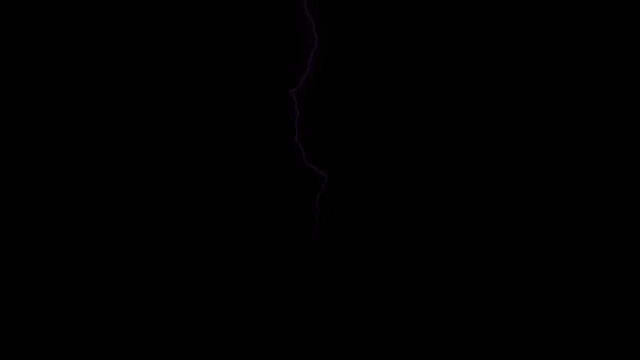 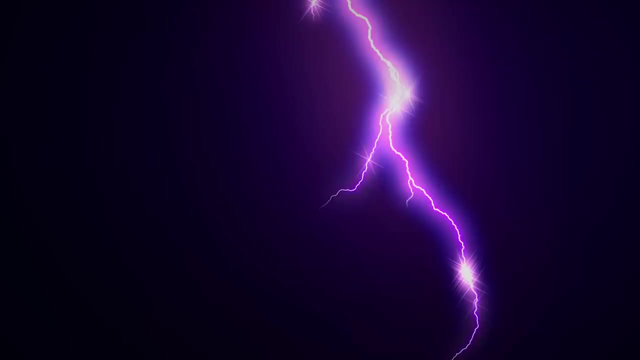 video. Let's go back and see how Maxwell's law shook classical mechanics. Are you ready for the revolution? One of the peculiarities of classical electromagnetism is that it is difficult to reconcile with classical mechanics, but it is compatible with special relativity. 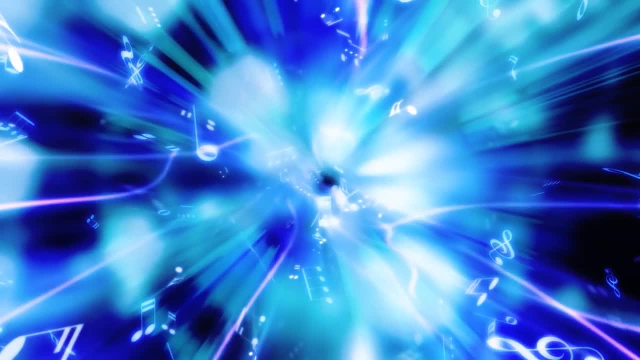 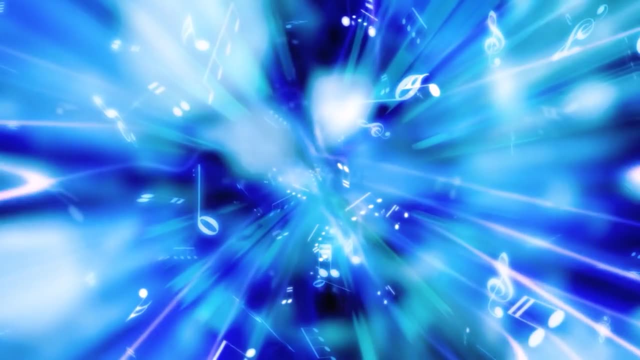 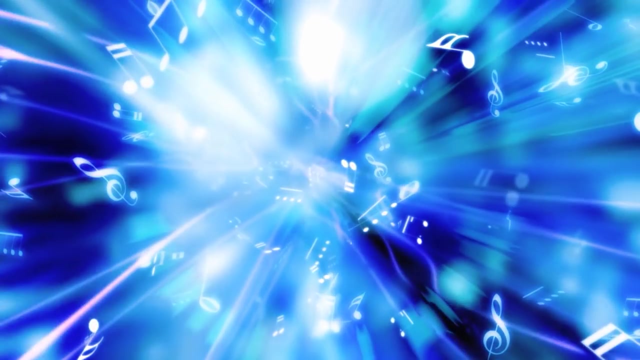 How? How is that possible? It has something to do with the changing of the reference system. According to Maxwell's equations, the speed of light in a vacuum is a universal constant that is dependent only on the electrical permittivity and magnetic permeability of free space. 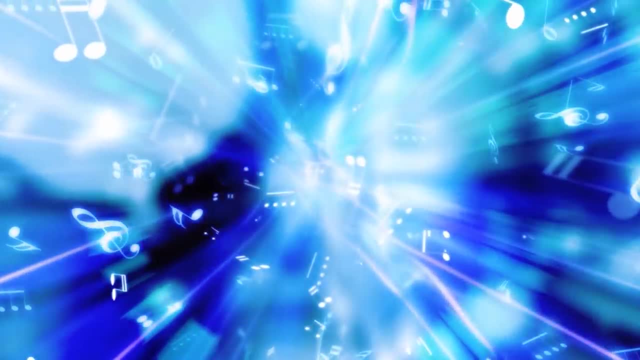 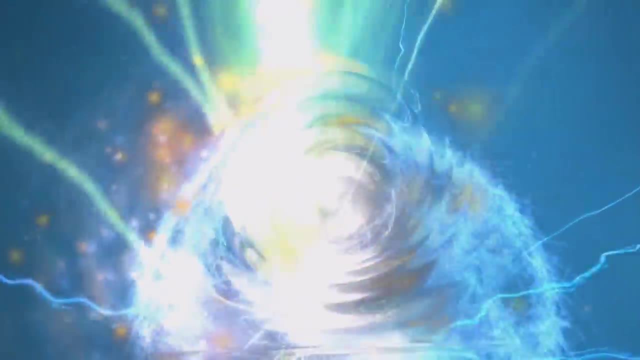 This violates Galilean invariance, a long-standing cornerstone of classical mechanics. One way to reconcile the two theories—electromagnetism and quantum mechanics—is to use quantum mechanics as the basis of quantum mechanics. Electromagnetism and classical mechanics was to assume the existence of a substance. 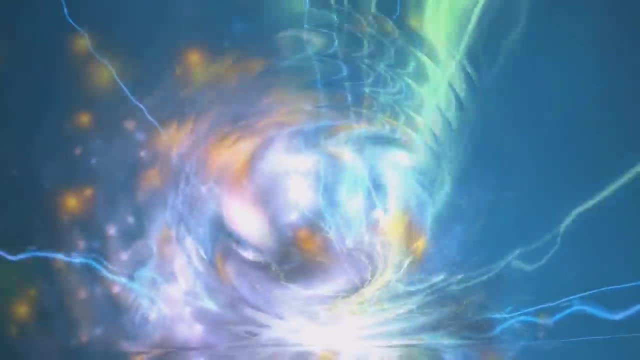 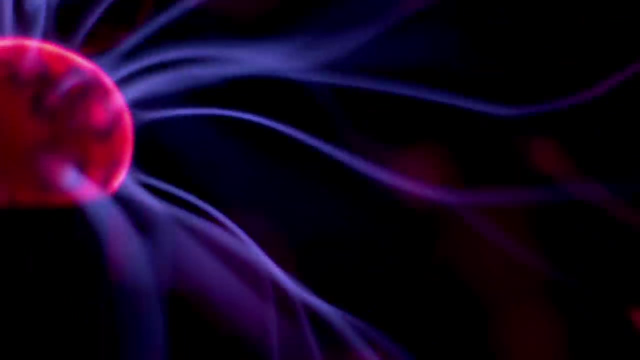 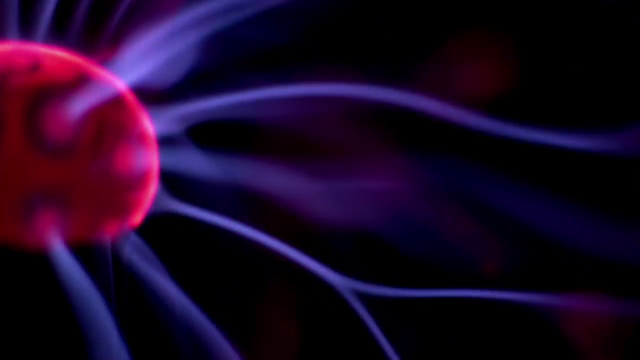 called luminiferous aether, through which the light propagates, But experimental efforts failed to detect the presence of the aether. One of the most famous experiments to prove or disprove the existence of the aether was the Michelson and Morley experiment. 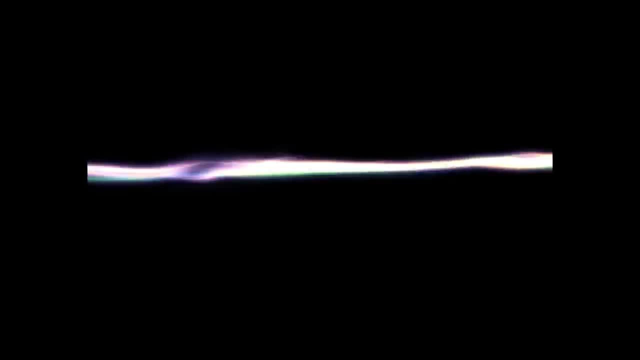 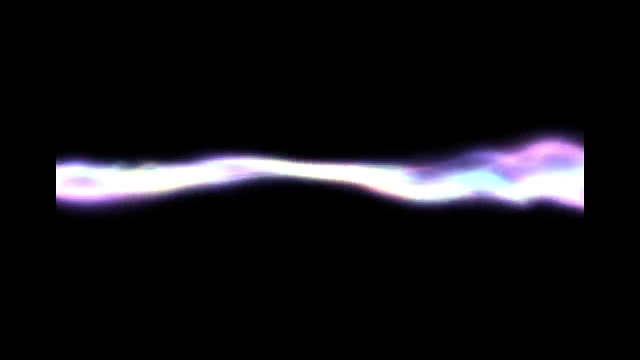 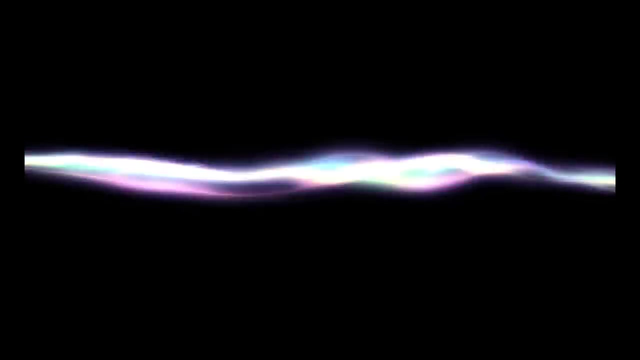 It was an attempt to detect the velocity of Earth with respect to the hypothetical luminiferous aether. The procedure depended on a Michelson interferometer, a sensitive optical device that compares the optical path lengths for light moving in two mutually perpendicular directions. Michelson reasoned that if the speed of light were constant with respect to proposed aether, 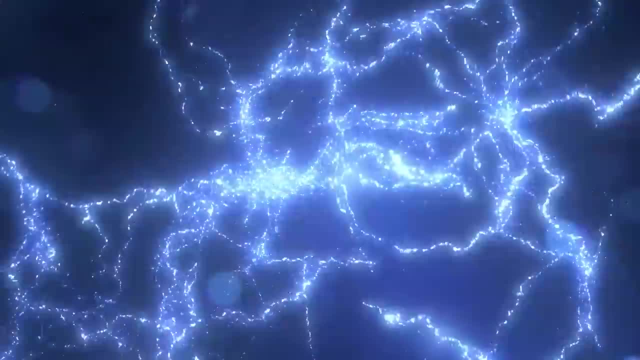 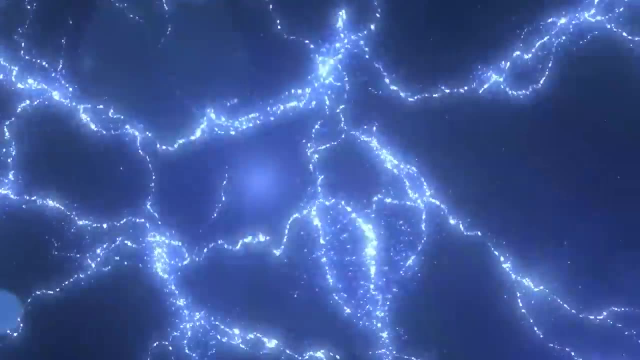 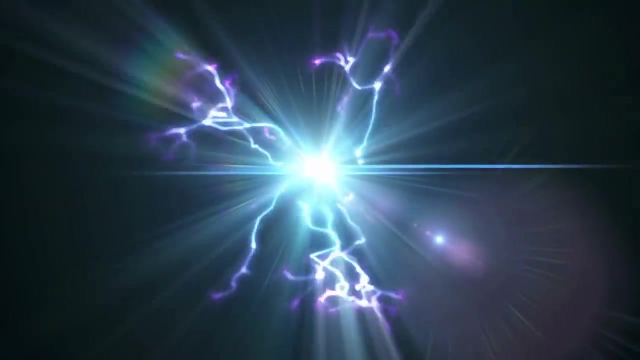 through which the Earth was moving. that motion could be detected by comparing the speed of light in the direction of the Earth's motion and the speed of light at right angles of the Earth's motion. No difference was found. This null result seriously discredited the aether theories and ultimately led to the 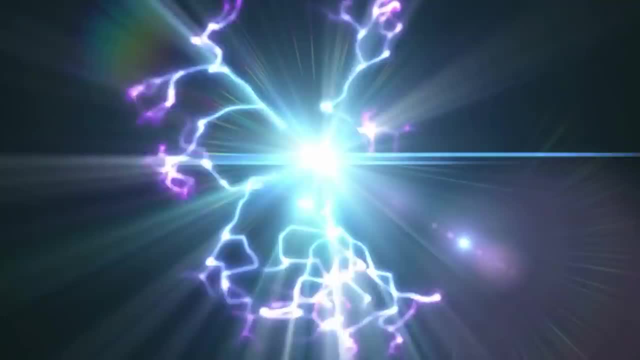 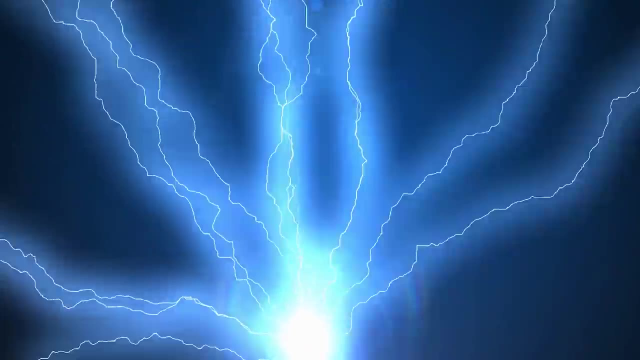 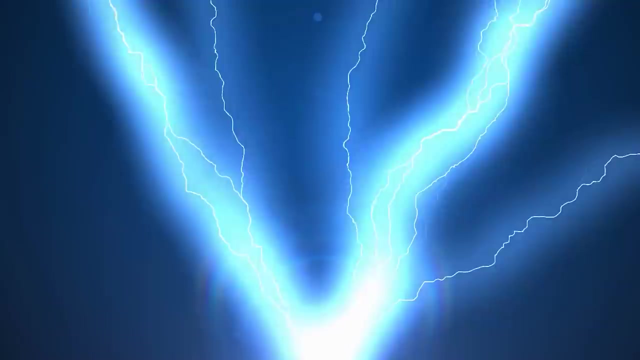 proposal by Albert Einstein in 1905 that the speed of light is a universal constant. After the important contributions of Hendrik Lorenz and Henri Poincaré in 1905, Albert Einstein solved the problem with the introduction of special relativity, which replaced the. 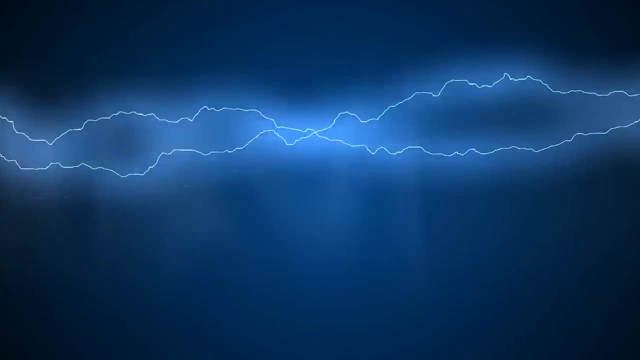 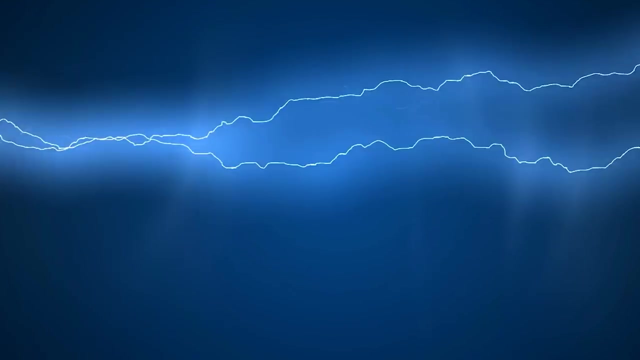 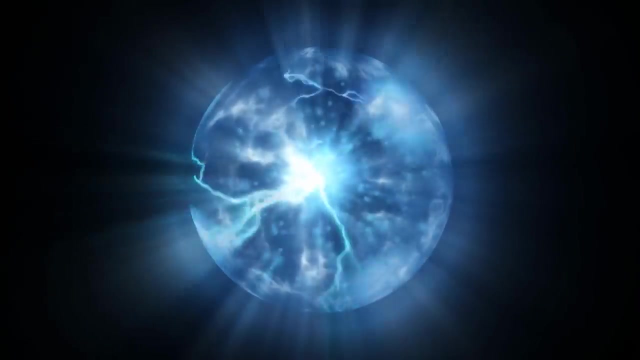 classical kinematics with a new theory of kinematics compatible with classical electromagnetism. For more information, see History of Special Relativity. In addition, relativity theory implies that in moving frames of reference a magnetic field transforms to a field with a non-zero electric component and, conversely, a moving 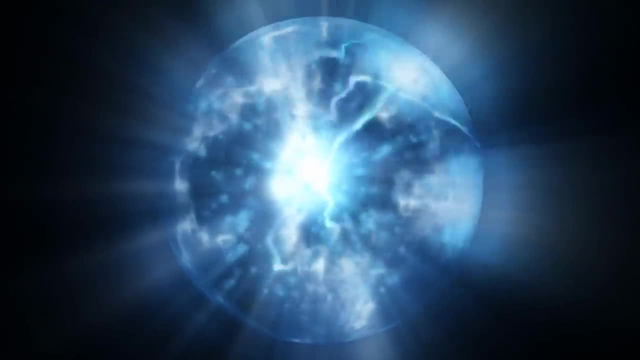 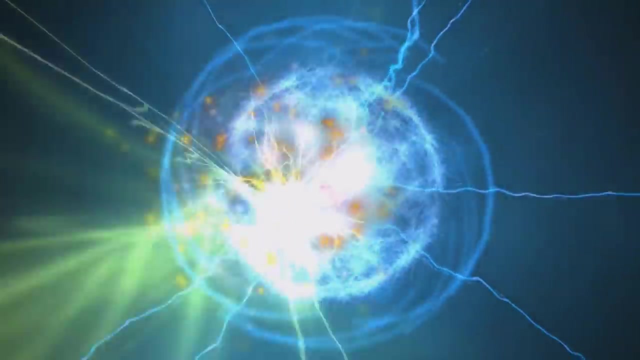 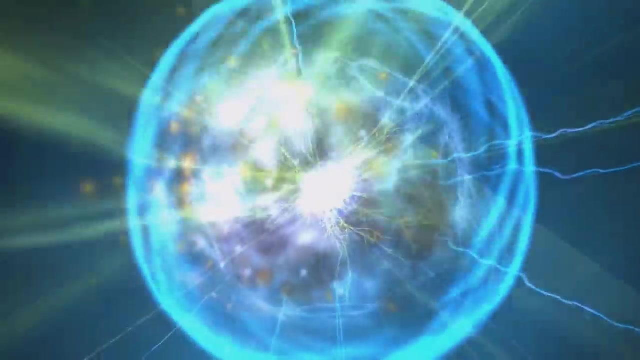 electric field transforms to a non-zero magnetic component, Thus firmly showing that the phenomena are two sides of the same coin, hence the term electromagnetism. For more information, see Classical Electromagnetism and Special Relativity and Covariant Formulation. 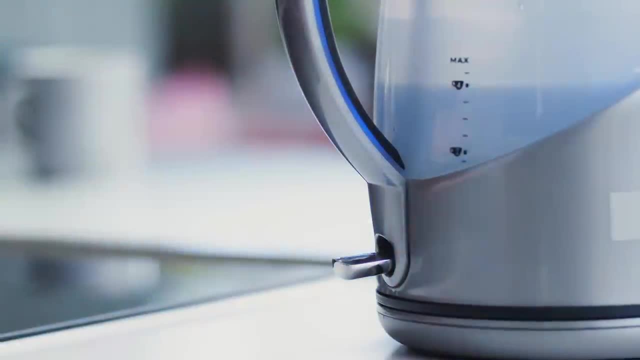 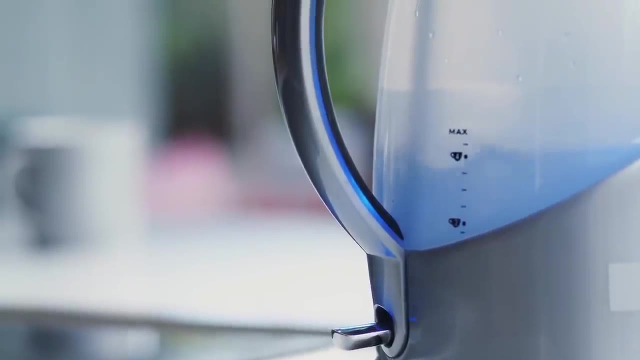 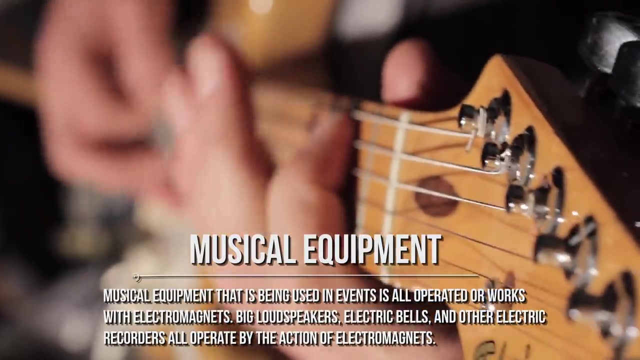 of Classical Electromagnetism. Before ending the video, we want to remind you that nowadays, electromagnetism-derived technologies are all around us. Here are some examples: Musical Equipment, Musical equipment that is being used in events, is all operated or works with electromagnets.